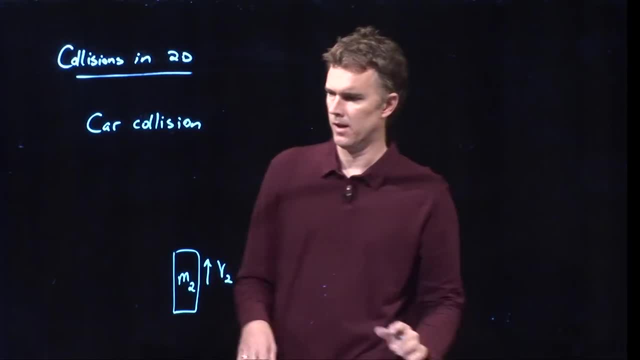 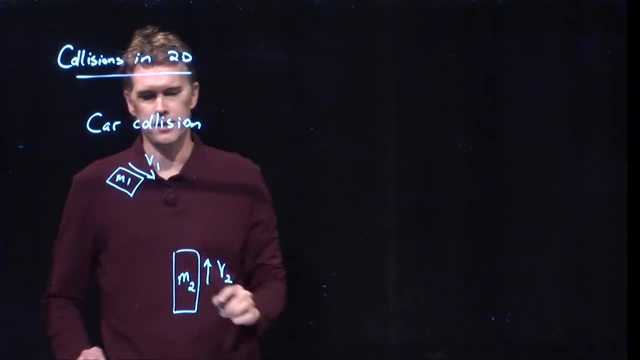 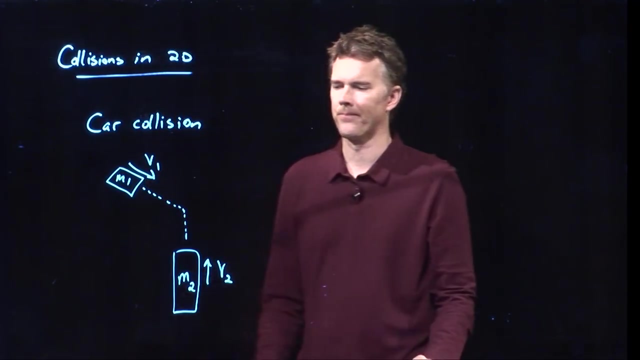 moving in this direction at speed v2. And then we have another car here that is mass m1. It's moving at speed v1. And these two things are going to come together and collide right there. And when they come together and collide, let's say they stick together. okay, This is a pretty 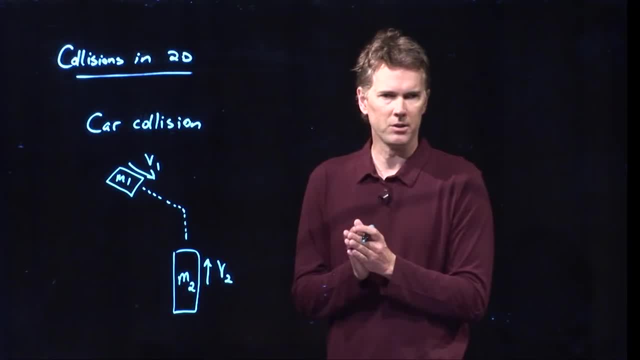 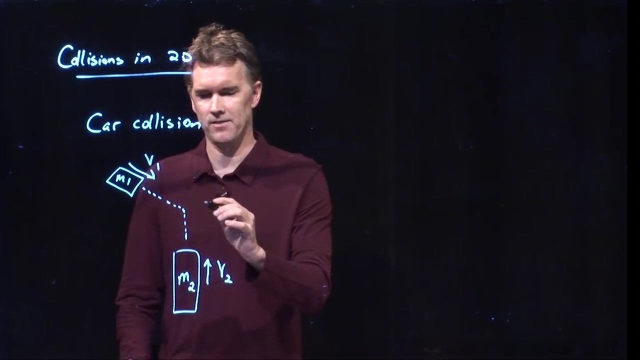 good approximation to what happens in a real car collision. okay, When cars collide they tend to sort of stick together because the bumpers get deformed, things bend, there's a whole bunch of energy lost in that collision, And so it is truly an inelastic collision. So after they collide, 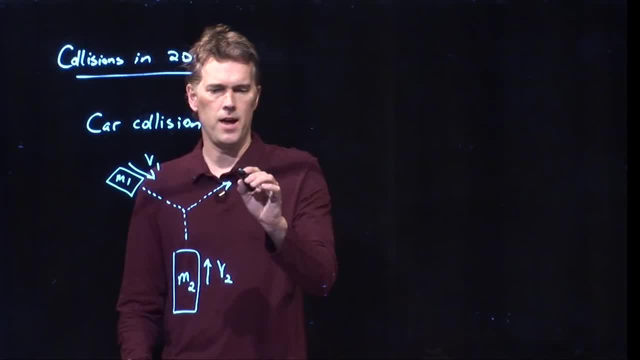 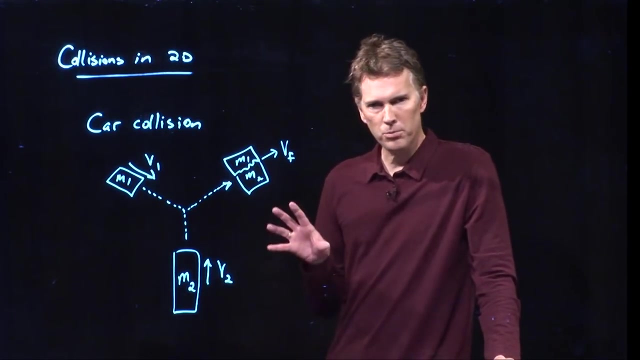 they're going to head off in some new direction And they are going to be stuck together. There's car one, There's car two. They are stuck together And they're moving at some final speed. v sub f. So this is what it looks like in general, And 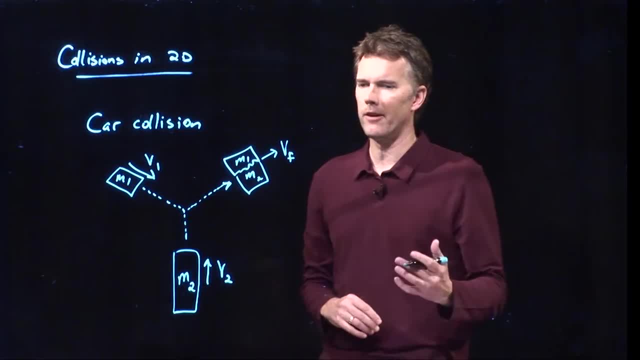 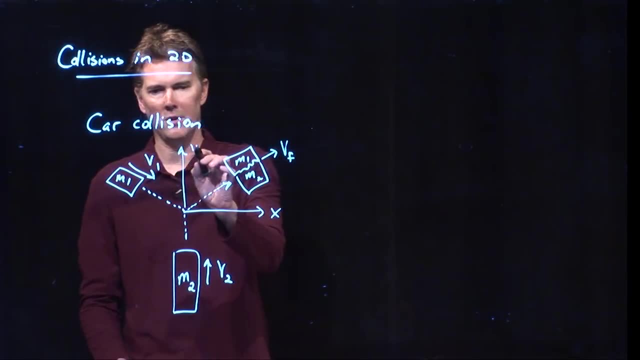 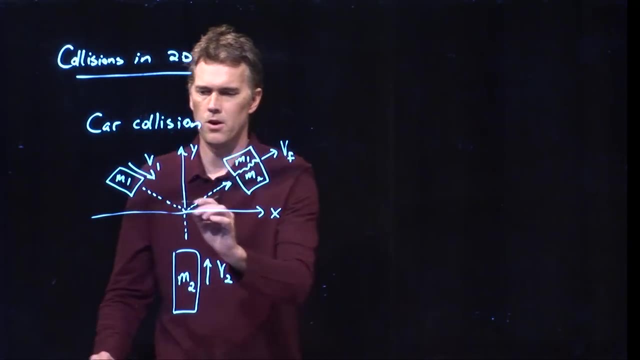 whenever you draw something in general like this, you should always identify a coordinate system. So it makes sense to use this as our x and use this as our y, And if that's the case, then we need to identify some angles. Let's call this angle phi And just. 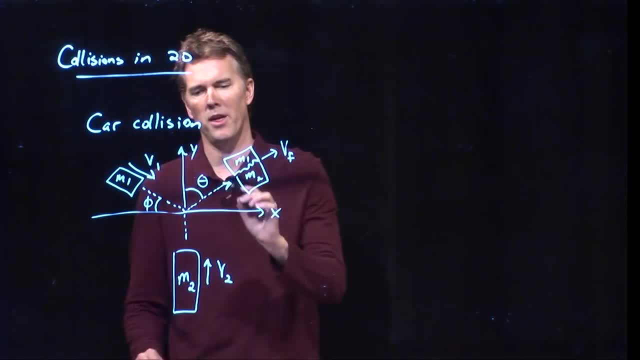 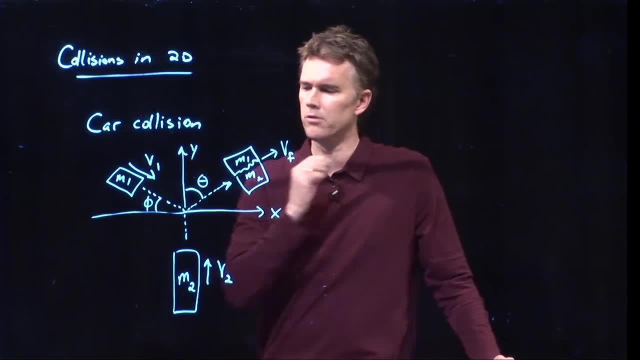 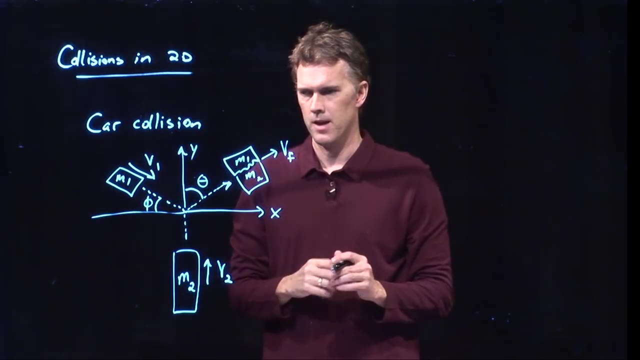 for kicks. let's call this angle theta. okay. Usually we write theta relative to the x-axis, But just as an example, let's use that as our theta, okay? So this is the before picture. This is the after picture. 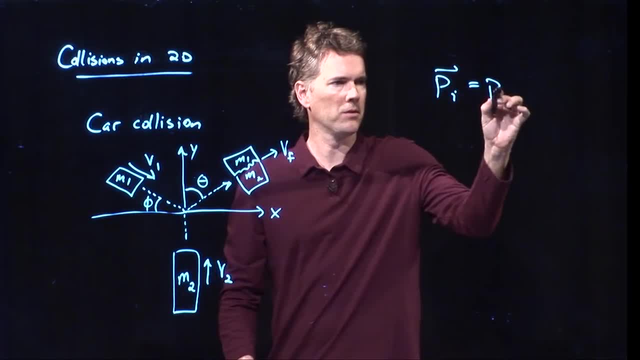 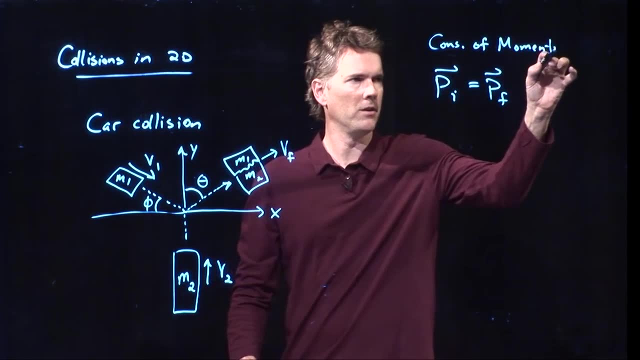 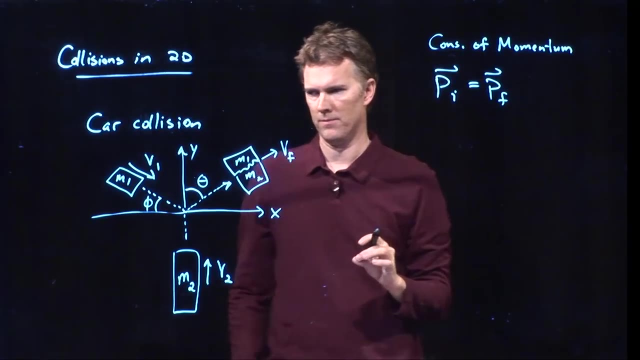 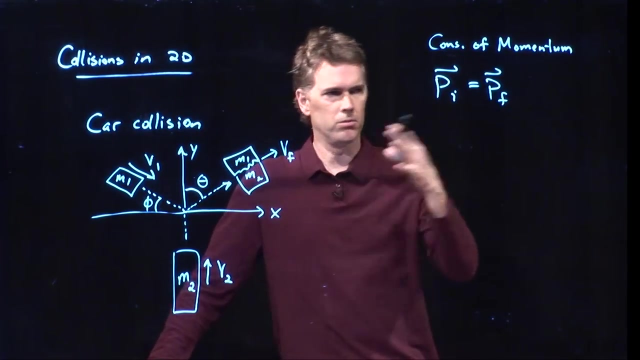 And now we can write down conservation of momentum. It tells us that p initial is equal to p file, And those are vectors And each one has two elements in it. Okay, We have an m1 and an m2 on the left side. We have an m1 and an m2 on the right side. We have x components. 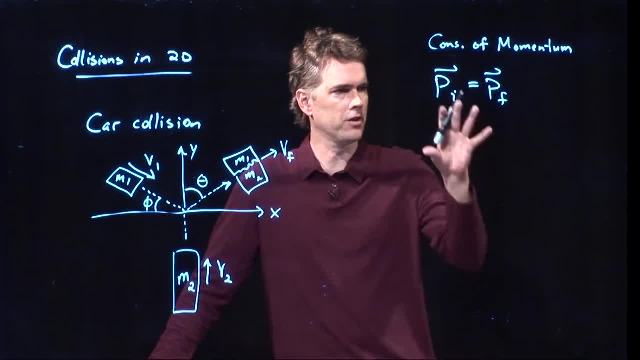 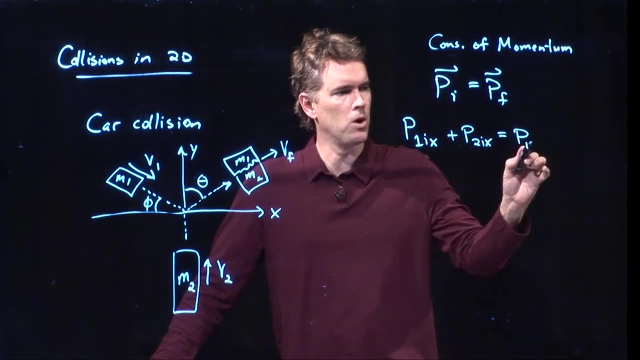 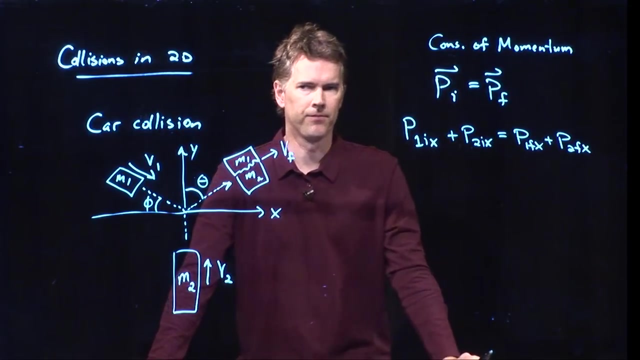 We have y components. We have a lot in there, So let's expand this a little bit. Let's do the x components first. P1.. P1, initial in the x plus p2, initial in the x equals p1 final in the x plus p2, final in the x. 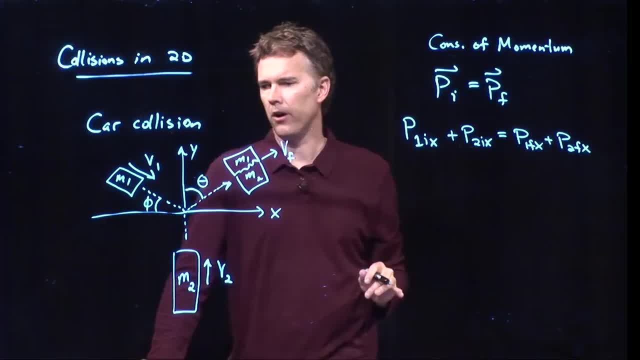 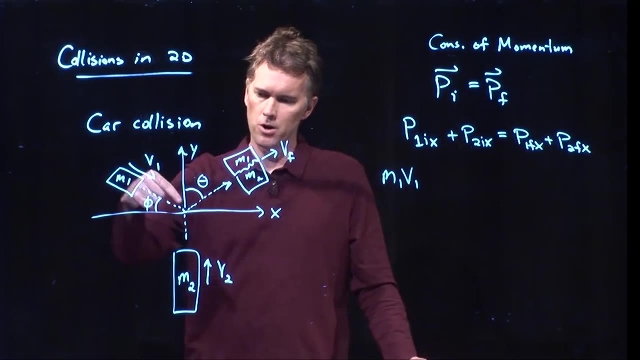 And let's do this part explicitly. So m1, v1 is the momentum of the initial guy, but we want the x component of it Right. It's coming down at this funky angle. It's partially in the x, It's partially in the y. 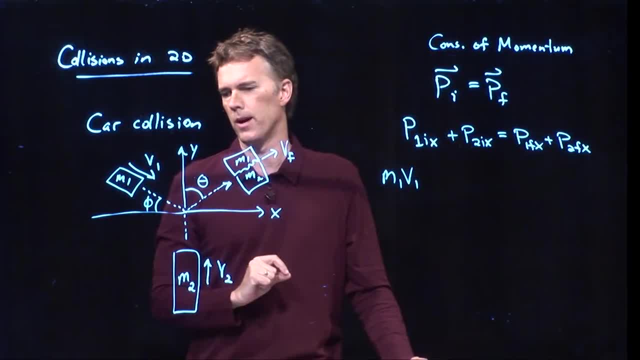 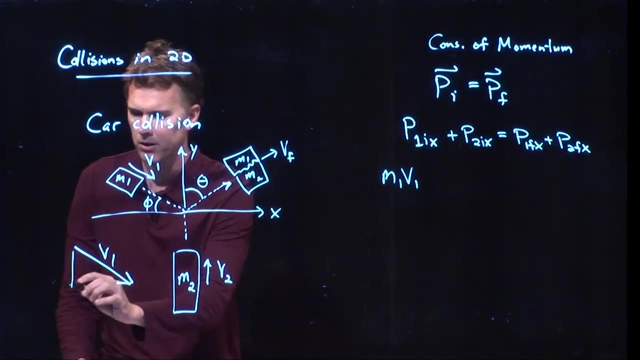 So we have to worry about what is in the x direction. So when I think about this velocity vector right there, v1, what can I say? Well, v1 is kind of coming down like that And that's going to have some component in the y and some component in the x. 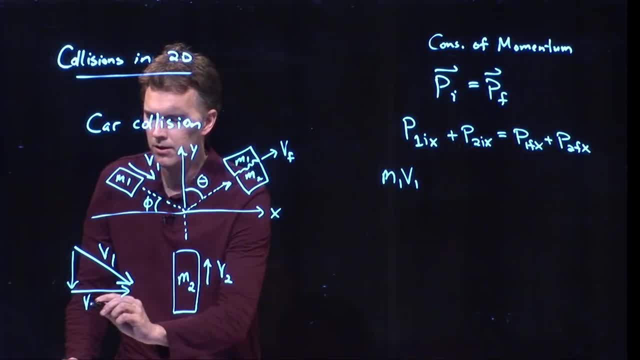 And so this component is going to have some component in the x, And so this component is going to have some component in the y and some component in the x. side of the triangle is the x, this side of the triangle is the y, and if that is, 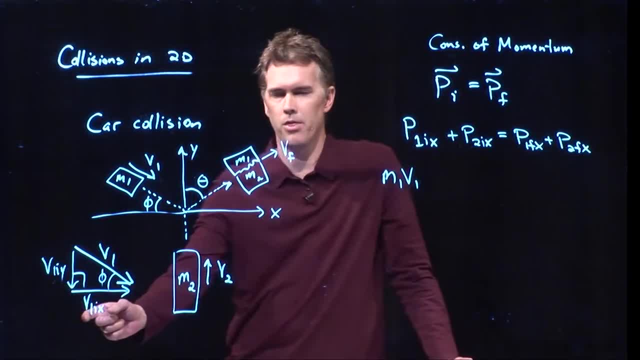 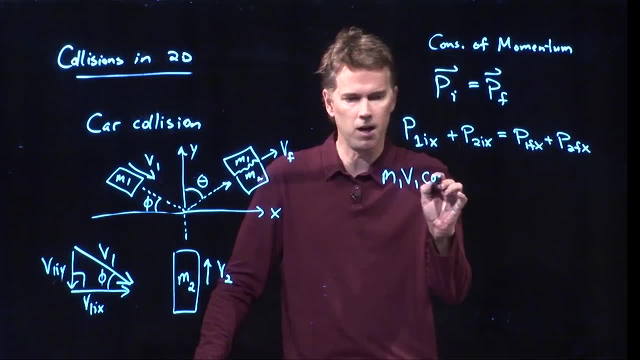 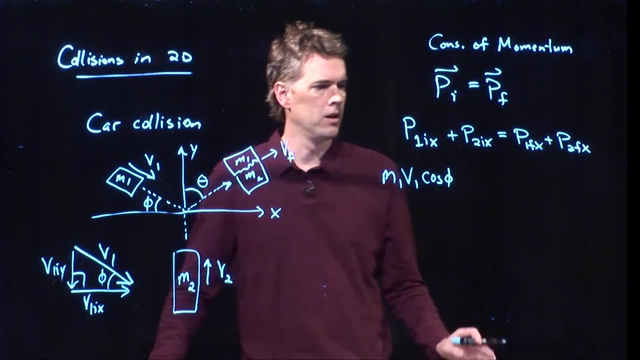 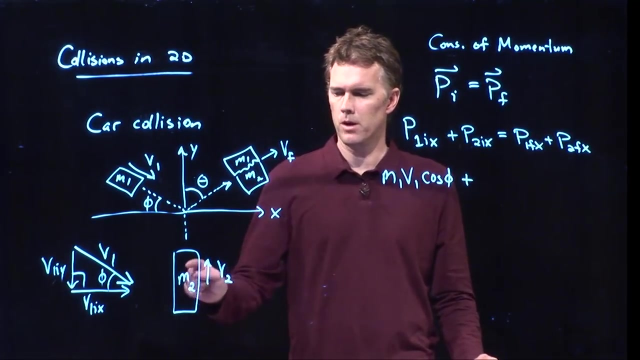 angle phi, and that's our right angle, then I know that this one is going to be cosine. So right here I need a cosine of phi. That's this first term p1 initial on the x. What about p2 initial in the x? What is the momentum of this guy in the? 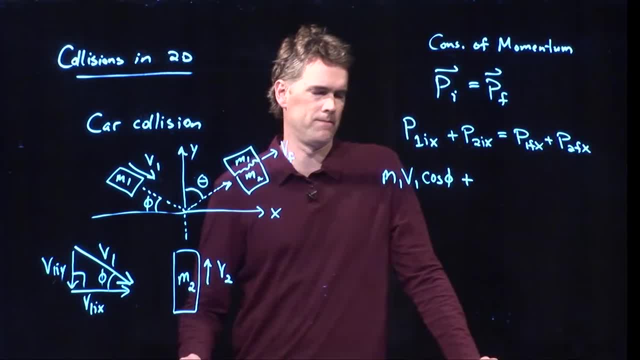 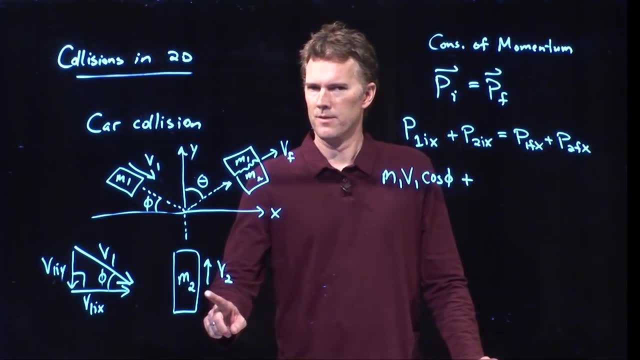 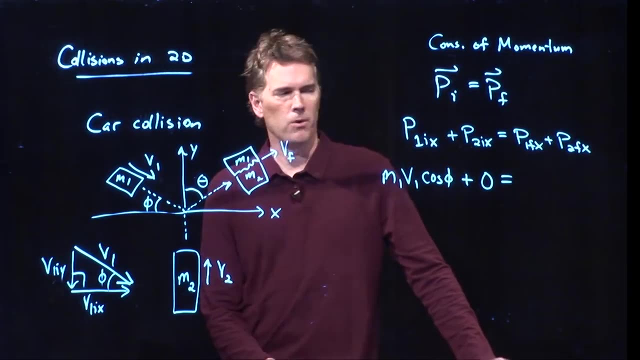 x direction. Chris, what do you think It's gonna be? mv sine theta. Okay, we're looking at this one right here. Sorry, the x is zero. X is zero, perfect, Very nice. Okay, now let's worry about the right side of this equation. 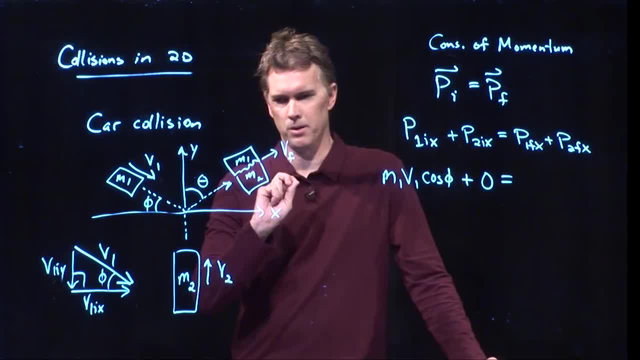 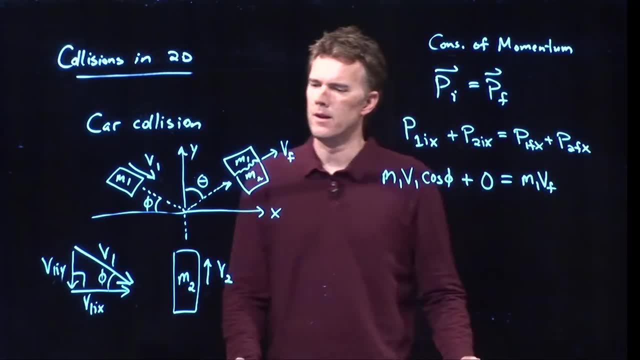 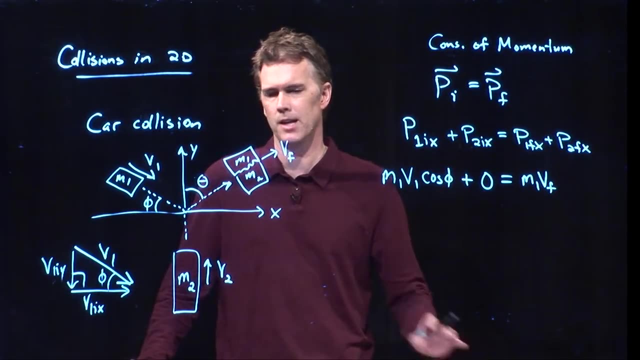 Well, I, Yes, I- can still treat these as independent particles, And so I can write this as m1 times v final. And now I have to figure out what the x component of this thing is. Let's take a look at this v final. 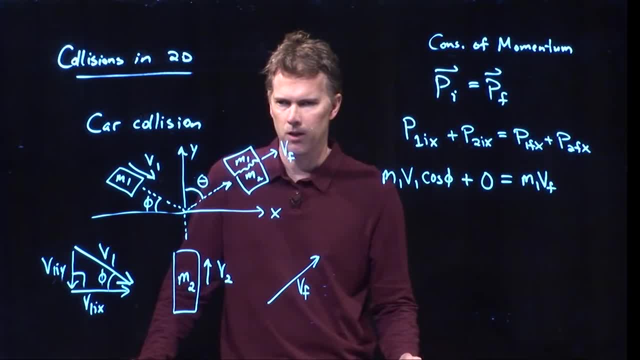 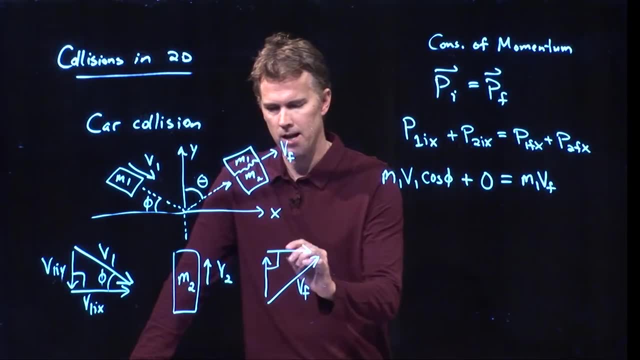 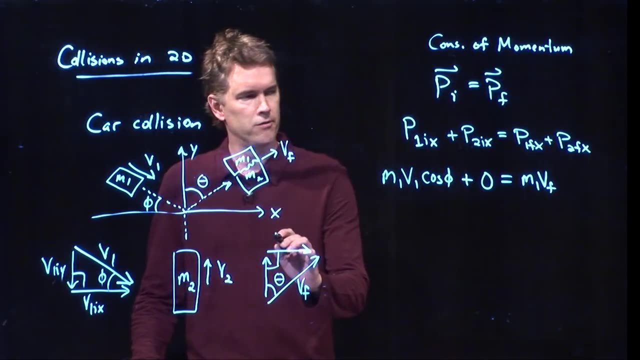 v final is heading up in that direction. That is composed of two things: vertical and horizontal. This is my right angle. This is the angle that we defined as theta. So this is going to be v final times, what It's going to be sine of theta. 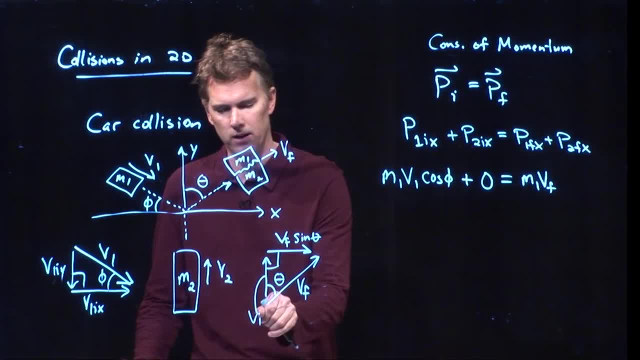 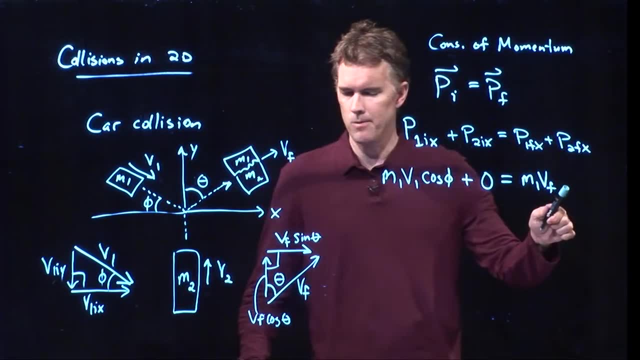 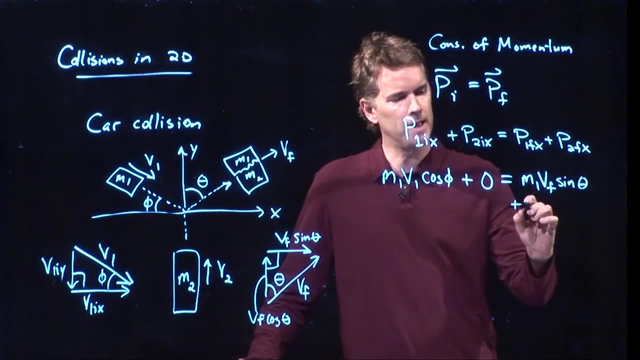 And this side over here is v1 cosine, Sorry, v final cosine theta. So on this right here I want v final sine theta, And then we have to add p2, but that's just m2 v final sine theta. And so on this right side we can in fact combine the two. 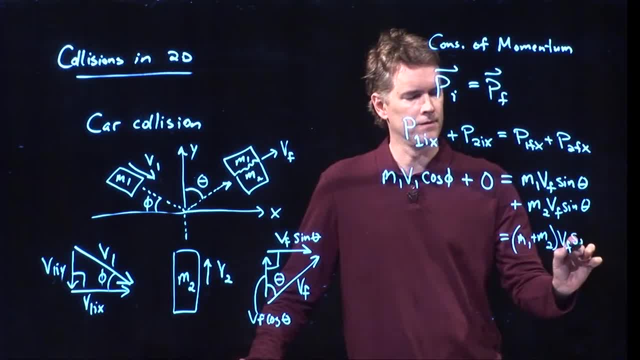 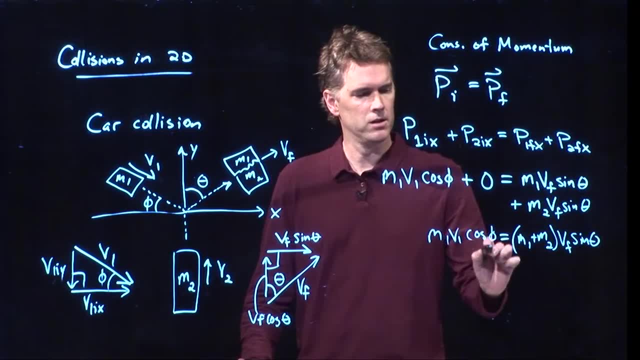 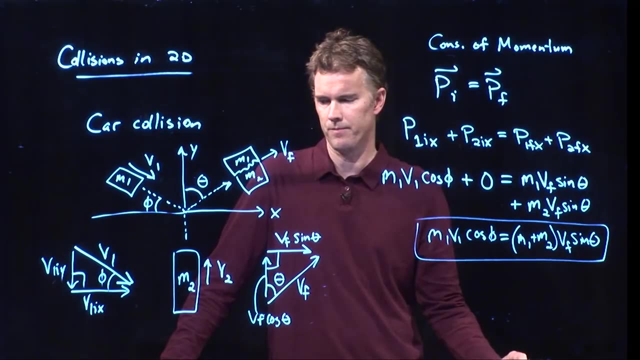 which makes sense. They're stuck together. Okay, so let's rewrite this equation: m1 v1 cosine phi equals m1 plus m2 v, final sine theta. Okay, Everybody okay with that part. so far, We're just looking at the x component now. 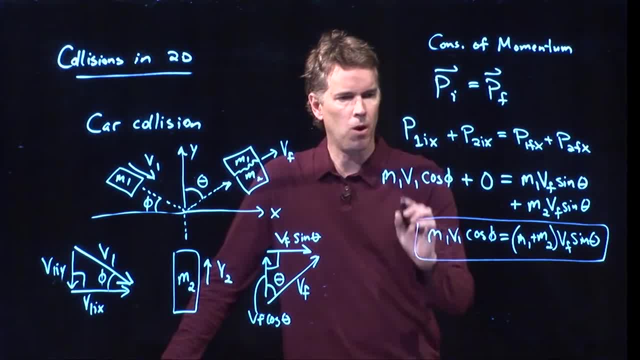 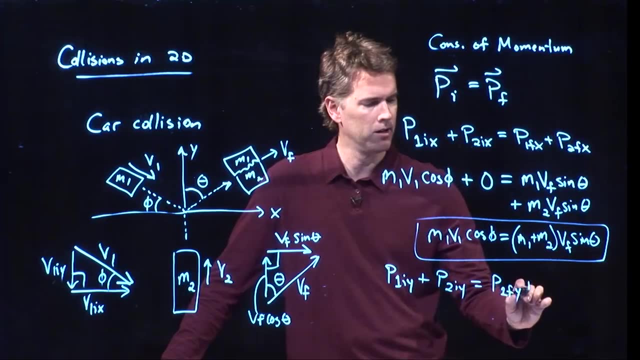 Okay, let's deal with the y component. The y component is going to look very similar to this. We're just going to change the x's to y's: p1 initial y plus p2 initial y equals p1 final y plus p2 final y. 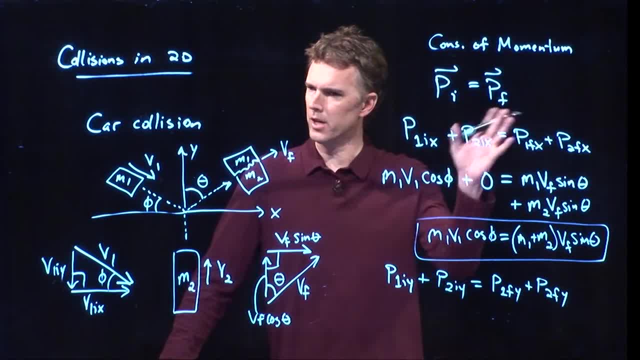 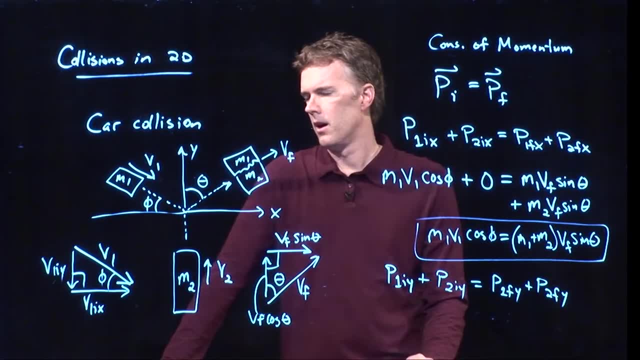 Okay, It's really the same equation. we just changed all the x's to y's And now we need to think about p1, initial in the y. All right, m1, v1,. we know that's got to be in there somewhere. 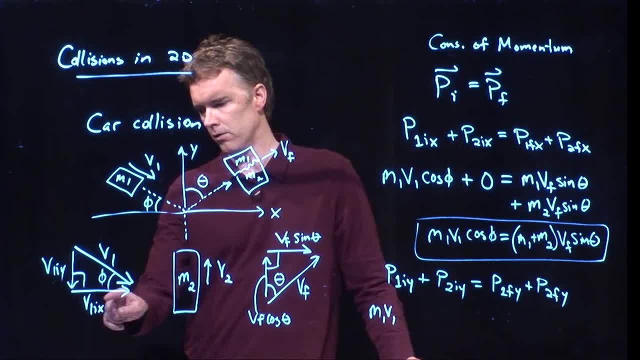 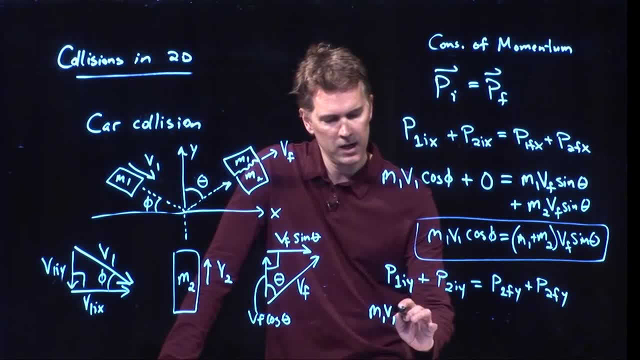 We used cosine before, so we probably want to use sine. That makes sense. That's this side of the triangle right, And sine is, let's see, Sine of theta. Okay, Sine of phi right. That was our angle. 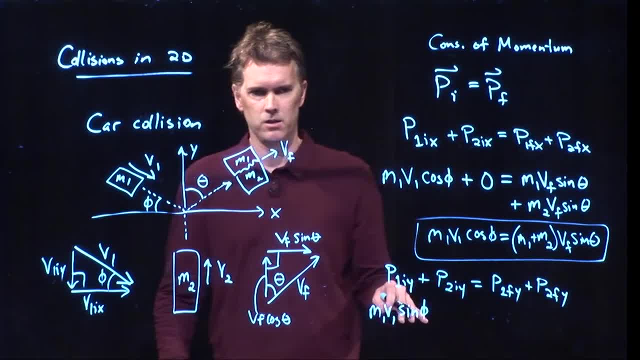 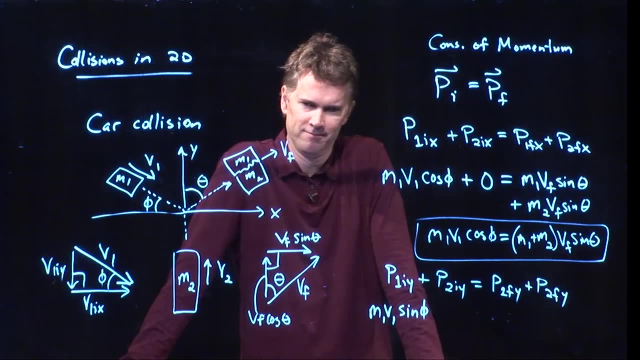 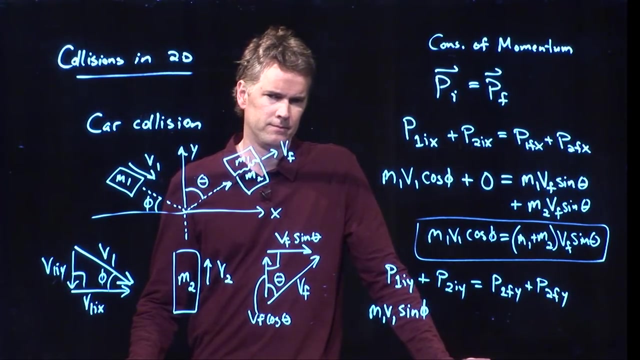 Okay, That looks pretty good. Is there anything else I want to add to this? Anything else I should put in here? Abdulaziz, Grab the mic. Anything else I want to put into this first statement right here? Okay, I actually don't know. 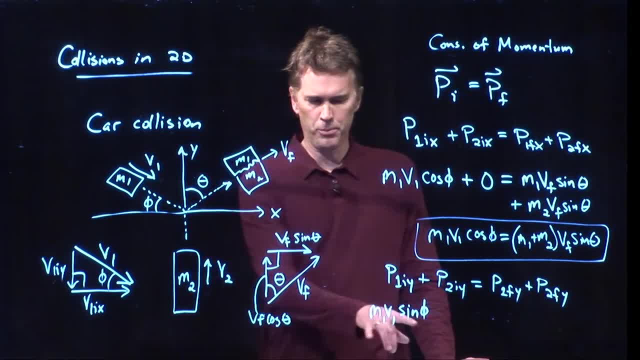 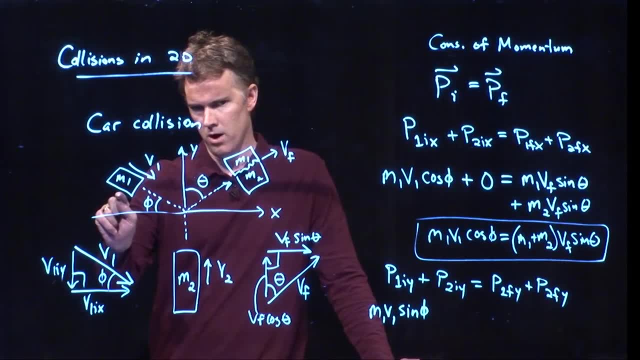 Okay, Well, it looks pretty good. right, We used the cosine before, so we're going to use the sine. But is this car m1, is this heading in the positive x direction or the negative x direction? It's the negative direction, so we should add a negative.